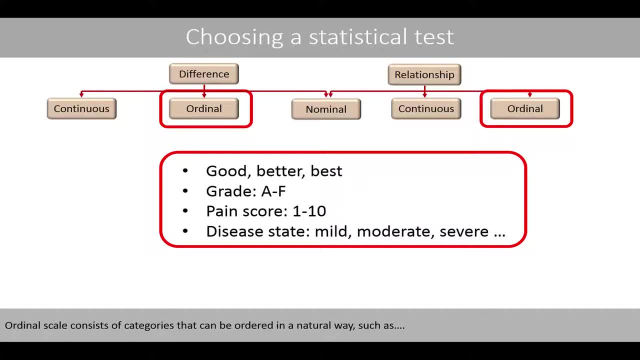 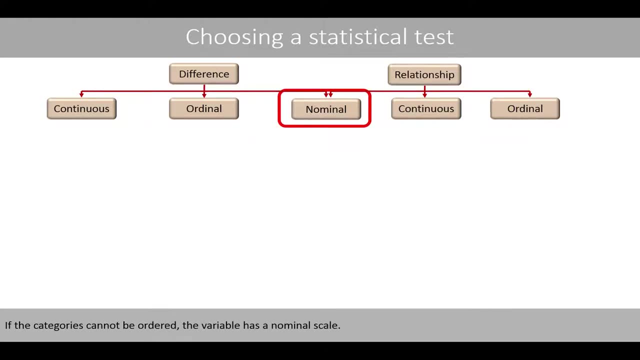 Ordinals scale consists of categories that can be ordered in a natural way, such as good, bad or best, the grades A to F, pain score between 1 and 10, and the disease states mild, moderate and severe. If the categories cannot be ordered, the variable has a numeral scale. 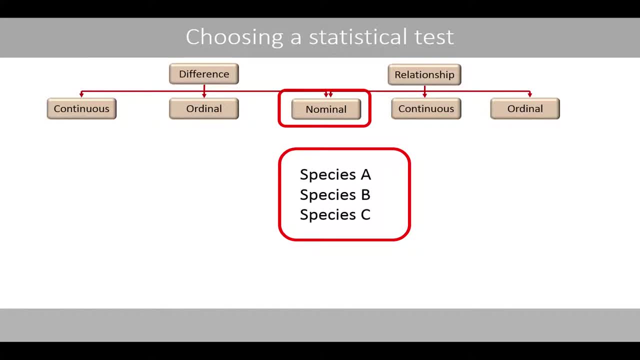 If the categories cannot be ordered, the variable has a numeral scale. For example, the species A, B and C are on a numeral scale, as well as the colors blue, red, orange and green. And the variable gender is also on a numeral scale, where we have the categories men and women. 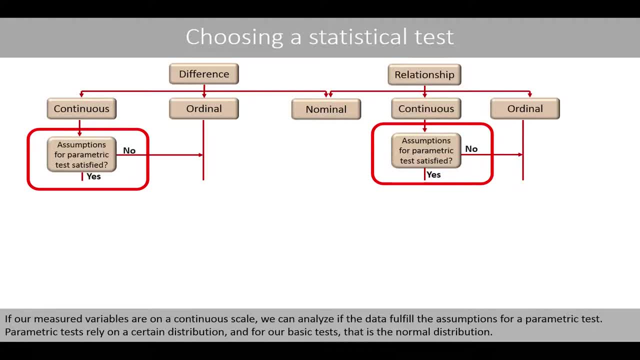 If our measured variables are on a continuous scale, we can analyze if the data have fulfilled assumptions for a parametric test. Parametric tests rely on a certain distribution And for our basic tests, this is the normal distribution. Since parametric tests generally have a higher statistical power than non-parametric tests, we should select a parametric test if we fulfill the assumption of normality. 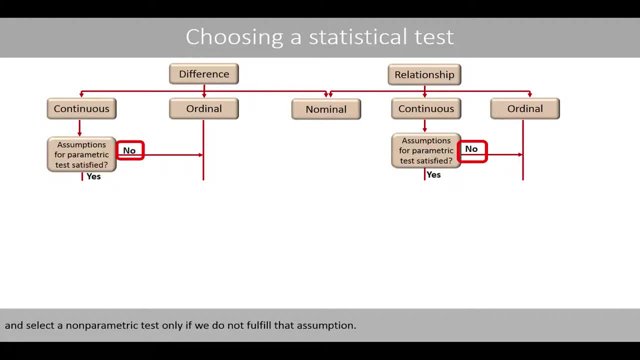 And select a non-parametric test only if we do not fulfill that assumption. If our measured variable appears to be normally distributed, we can be quite confident that we fulfilled the normality assumption. If our measured variable appears to be normally distributed, we can be quite confident that we fulfilled the normality assumption. 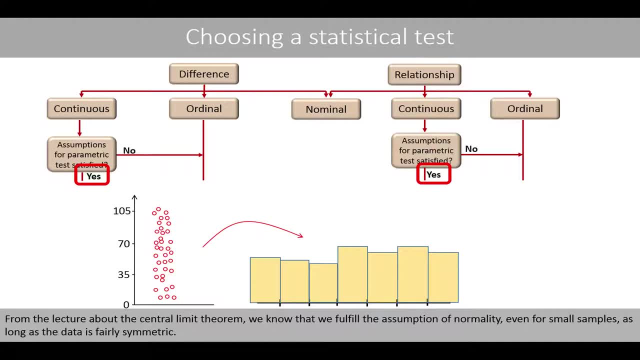 From the lecture about the center limit theorem, we know that we fulfill the assumption of normality even for small samples, as long as the data is fairly symmetric. If the distribution is skewed, we need a larger sample size- generally bigger than 30, to fulfill the assumption of normality. 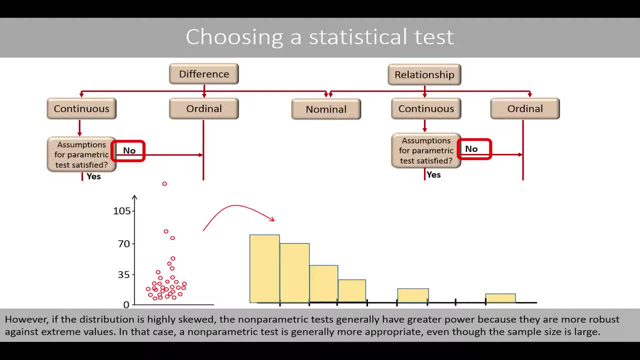 However, if the distribution is highly skewed, the non-parametric tests generally have a greater power. However, if the distribution is highly skewed, the non-parametric tests generally have a greater power. However, if the distribution is highly skewed, the non-parametric tests generally have a greater power. 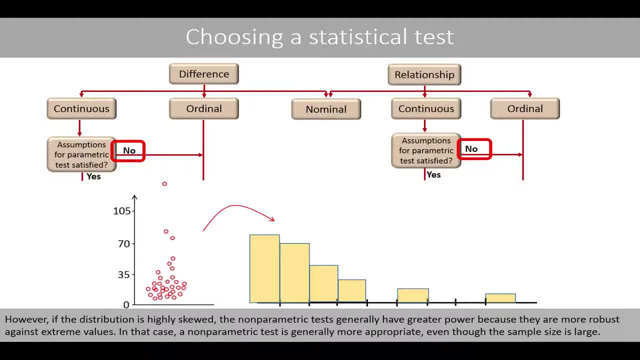 because they are more robust against extreme values. In that case, a non-parametric test is generally more appropriate, even though the sample size is large. Also, if most array data points appear to be normally distributed, but where extreme values are observed further away. 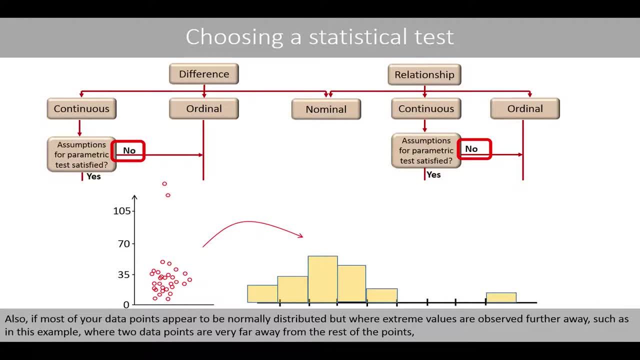 such as in this example, where two data points are very far away from the rest of the points. a non-parametric test is a better alternative, such as in this example where two data points are very far away from the rest of the points, because parametric tests are very sensitive to extreme values. 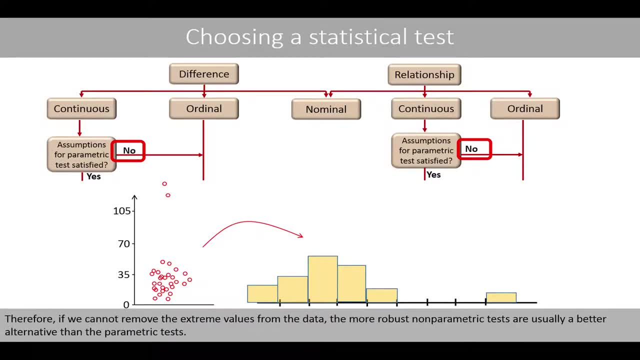 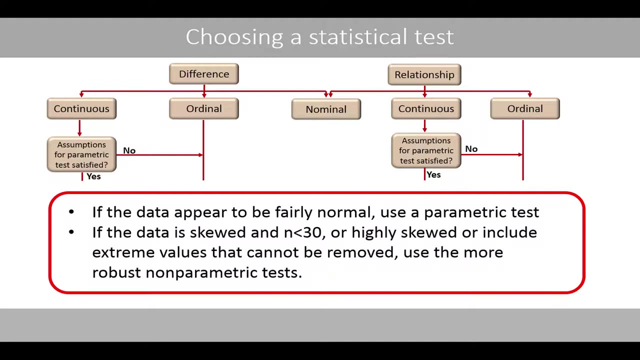 Therefore, if we cannot remove the extreme values from the data, then more robust non-parametric tests are usually a better alternative than their parametric tests. In conclusion, if the data appears to be fairly normal, use a parametric test If the data is skewed and the sample size is less than 30,. 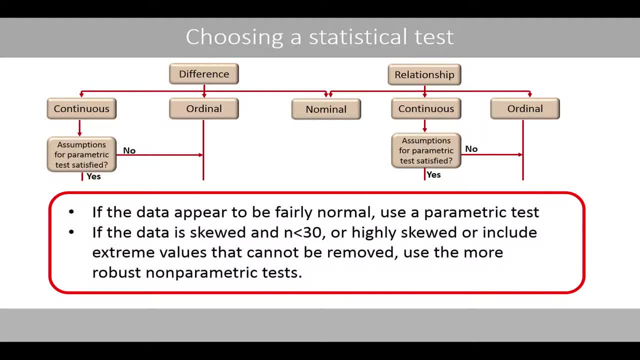 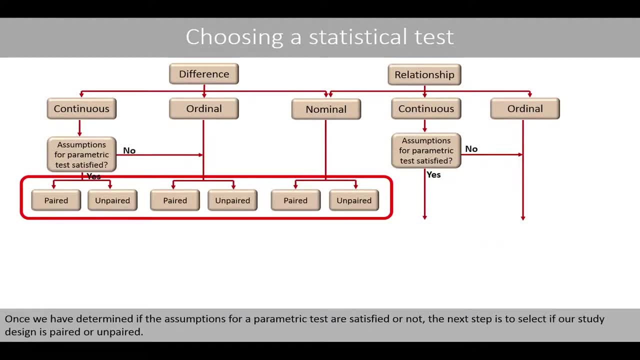 or highly skewed or include extreme values that cannot be removed, use the more robust non-parametric tests. Once we have determined if the assumptions for a parametric test are satisfied or not, the next step is to select if our study design is paired or unpaired. 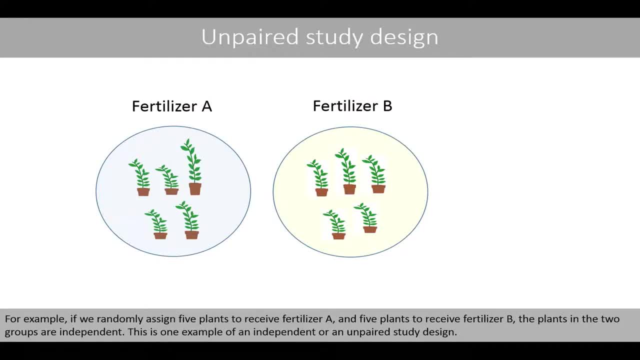 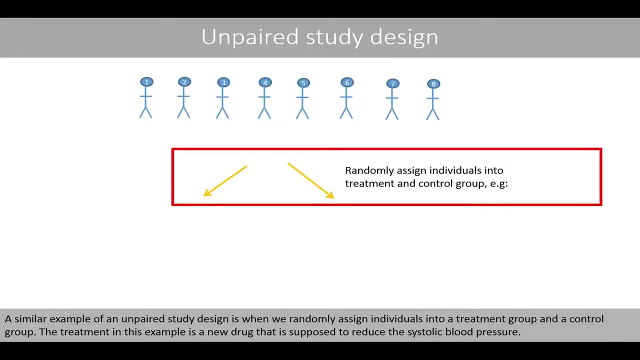 For example, if we randomly assign five plants to receive fertilizer A and five plants to receive fertilizer B, the plants in the two groups are independent. This is one example of an independent or unpaired study design. A similar example of an unpaired study design is when we randomly assign individuals. 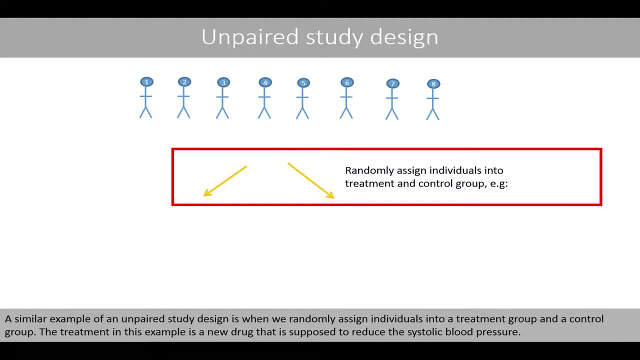 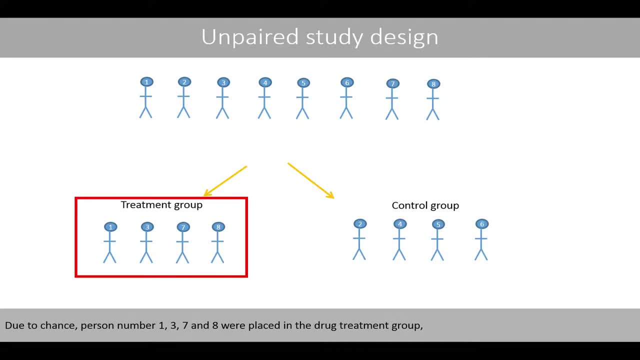 into a treatment group and a control group. The treatment in this example is a new drug that is supposed to reduce the systolic blood pressure. Due to chance, person number 1,, 3,, 7 and 8 were placed in a drug treatment group. 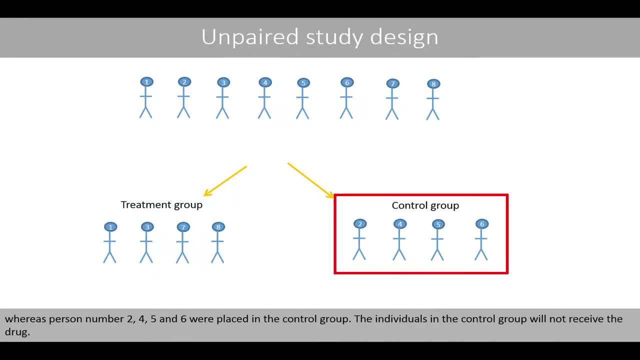 whereas person number 2,, 4,, 5 and 6 were placed in the control group. The individuals in the control group will not receive the drug. In this case, the two groups are independent and we therefore have an unpaired study design. 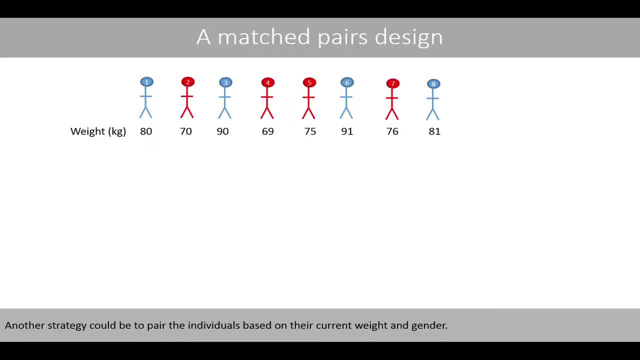 Another strategy could be to pair the individuals based on their current weight and gender. These numbers represent the body weight of the eight individuals before the treatment. We have four men and four women. For example, we could pair person number 1 and 8,. 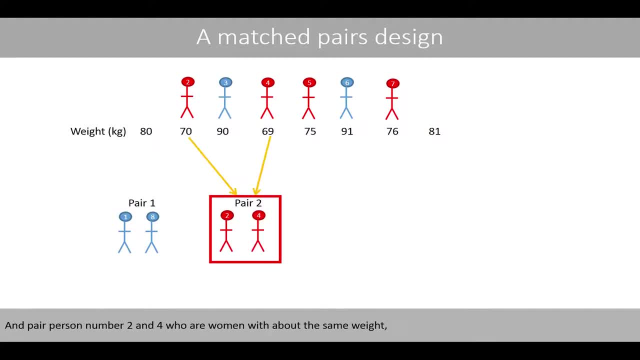 who have a similar weight and are both men, And pair person number 2 and 4,, who are both women with about the same weight. And then we pair person number 3 and 6. And finally, we pair the last two women. 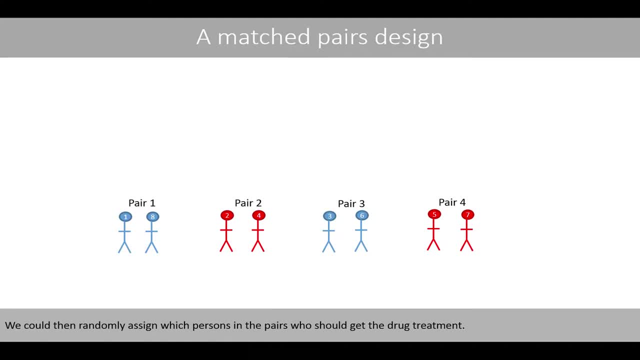 We could then randomly assign which persons in the pair who should get the drug treatment After some time. we checked the difference in the systolic blood pressure between the pairs. The advantage of this study design is that we reduced their variability, since we look at the difference between similar individuals. 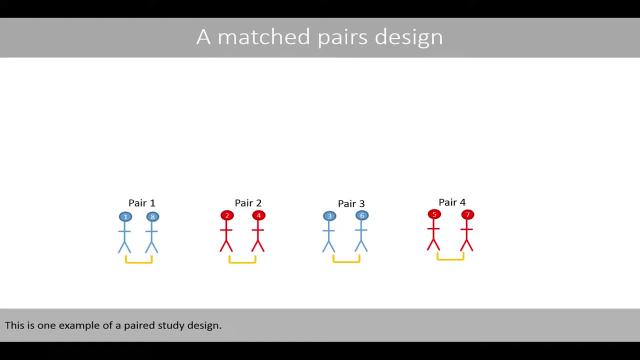 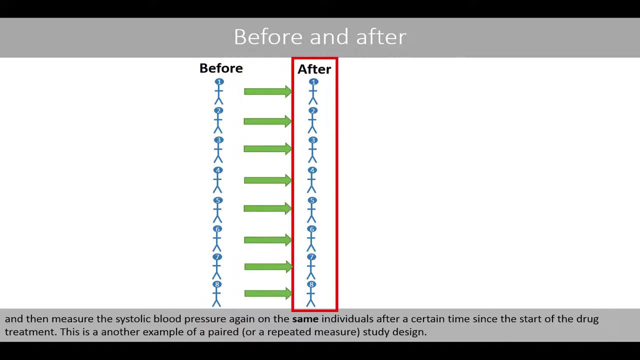 This is one example of a paired study design. Another common type of a paired study design is the so-called before and after studies. For example, we could measure the systolic blood pressure of all 18 individuals before taking the drug and then measure the systolic blood pressure again on the same individuals. 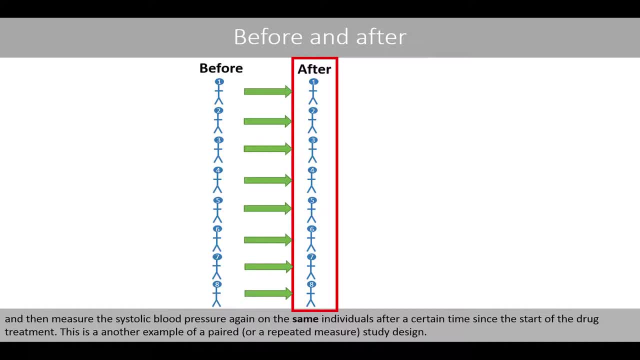 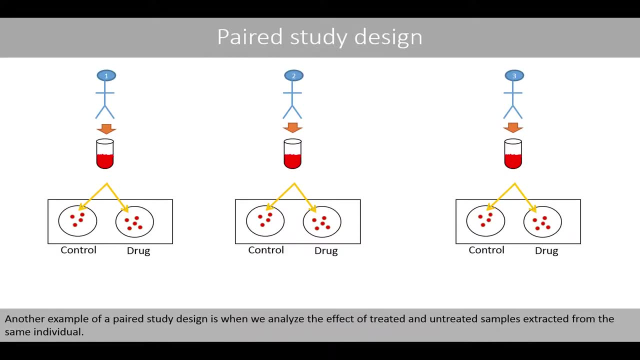 after a certain time since the start of the drug treatment. This is another example of a paired or repeated measured study design. Another example of a paired study design is when we analyze the effect of treated and untreated samples extracted from the same individuals, For example. 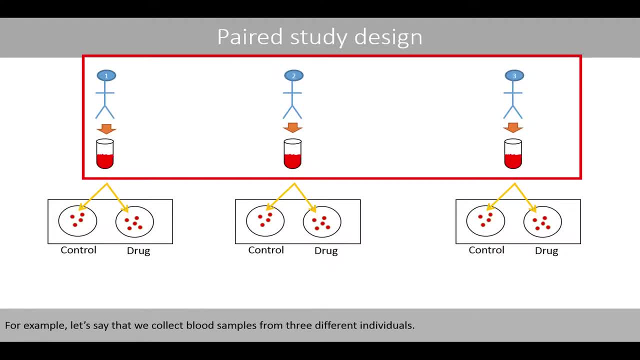 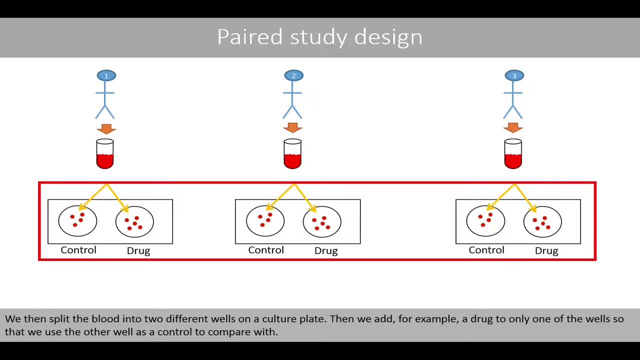 let's say that we collect blood samples from three different individuals. We then split the blood into two different wells on a culture plate. Then we add, for example, the drug to only one of the wells, so that we use the other well as a control to compare with. 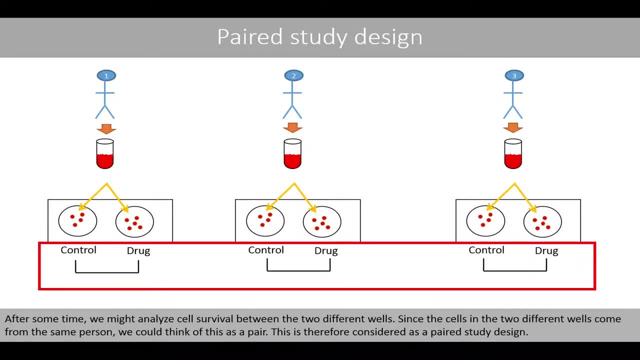 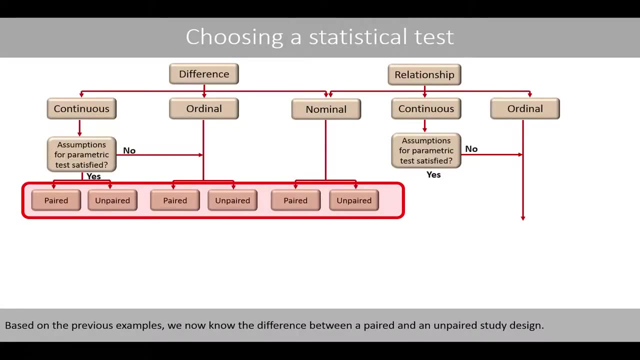 After some time, we might analyze cell survival between the two different wells. Since the cells in the two different wells come from the same person, we could think of this as a pair. This is therefore considered as a paired study design, Based on our previous examples. 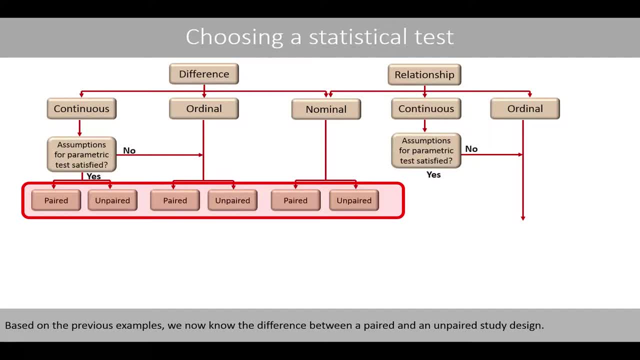 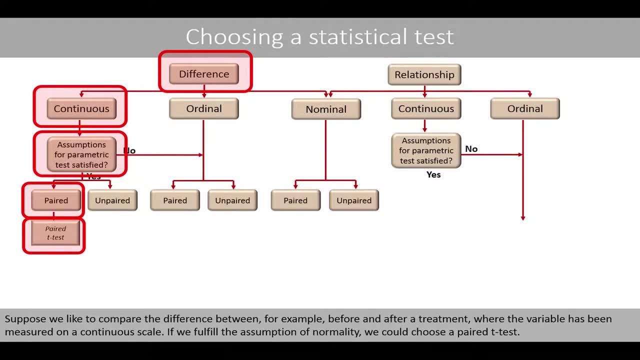 we now know the difference between a paired and an unpaired study design. Suppose we like to compare the difference between, for example, before and after a treatment where the variable has been measured on a continuous scale, If we fulfill the assumption on normality. 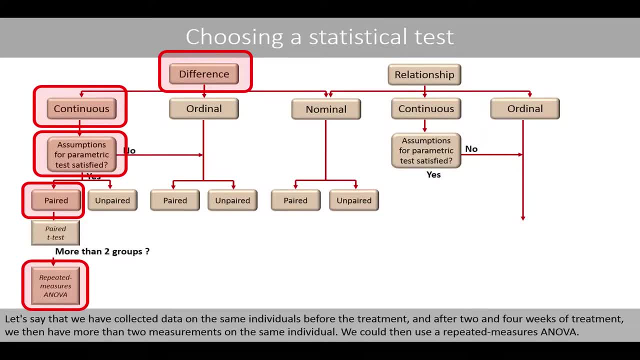 we could choose a paired t-test. Let's say that we have collected data on the same individuals before the treatment and after two and four weeks of treatment We then have more than two measurements on the same individual. We could then use a repeated measures analysis. 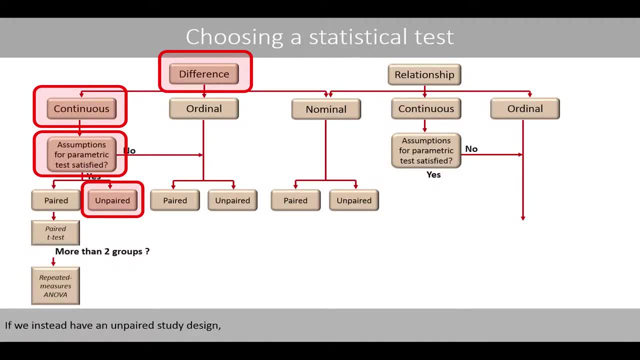 or ANOVA. If we instead have an unpaired study design, we could select an unpaired t-test if we like to compare two independent groups. Note that an unpaired t-test is also called an independent samples t-test If we like to compare more than two groups. 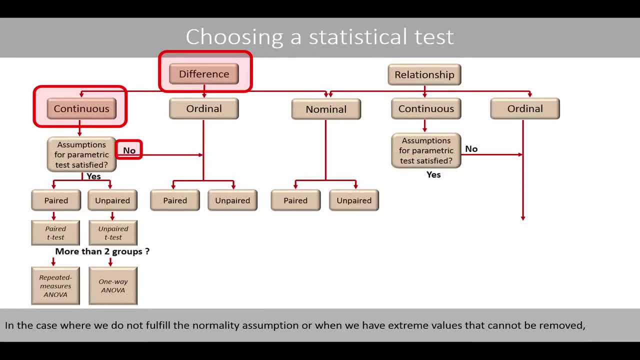 a one by ANOVA could be used In the case where we do not fulfill that normality assumption or when we have extreme values that cannot be removed, or if our measured variable has an ordinary scale. a non-parametric t-test is more appropriate. 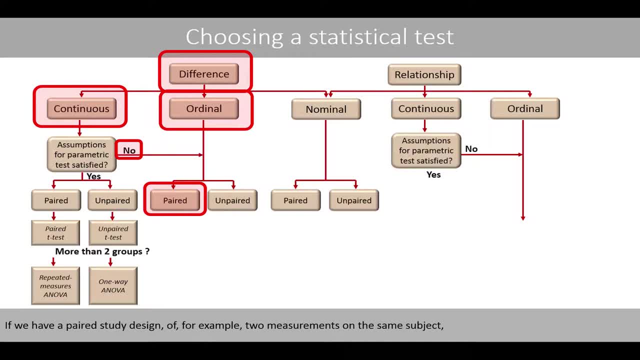 If we have a paired study design or, for example, two measurements on the same subject, we can select a Wilcoxon sign rank t-test if the data is on continuous scale and one of the differences have a symmetric distribution. If the data is on ordinary scale, 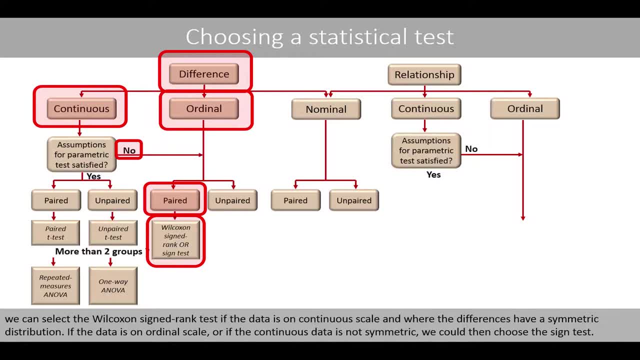 or if the continuous data is not symmetric, we could then choose the sign test. If we, for example, have more than two measurements on the same subject, we could use the Friedman t-test, which can be seen as the corresponding non-parametric alternative to the repeated measures ANOVA. 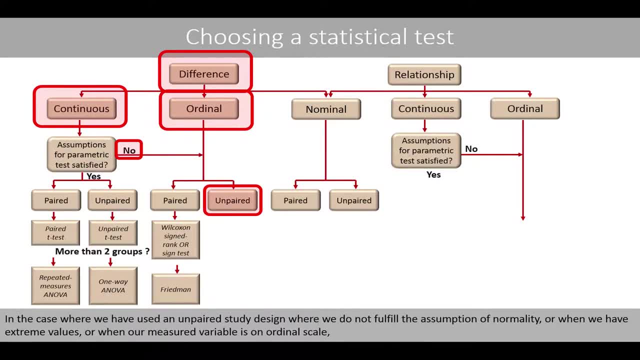 In the case where we have used an unpaired study design or we do not fulfill that assumption on normality, or when we have extreme values, or when our measured variable is on ordinary scale, we could select the Wilcoxon Mann-Whitney t-test. 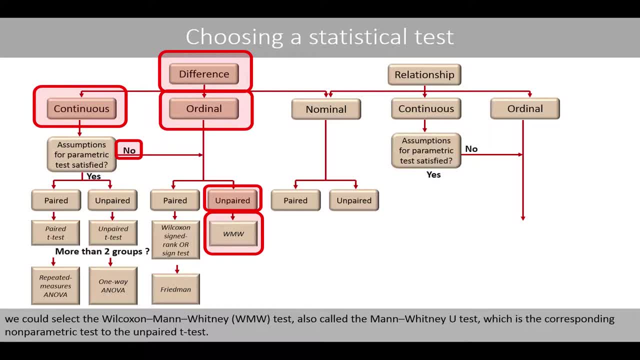 also called the Mann-Whitney U-test, which is the corresponding non-parametric test to the unpaired t-test. If we have more than two independent groups, we can use the Kruskal-Wallis test, which is the corresponding non-parametric test to the one by ANOVA. 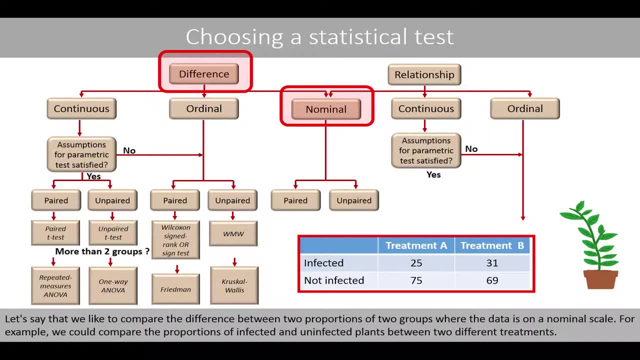 Let's say that we would like to compare the difference between two proportions of two groups where the data is on numeral scale. For example, we could compare the proportions of infected and uninfected plants between two different treatments. If the study design is unpaired, 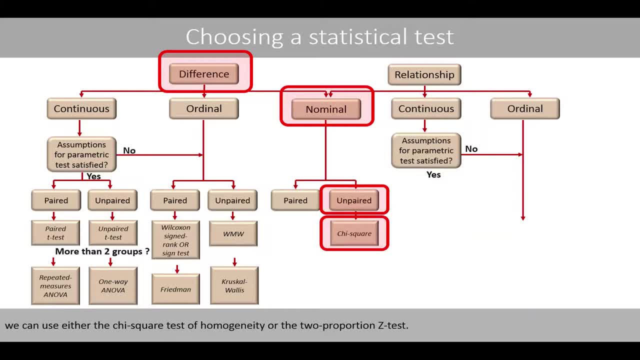 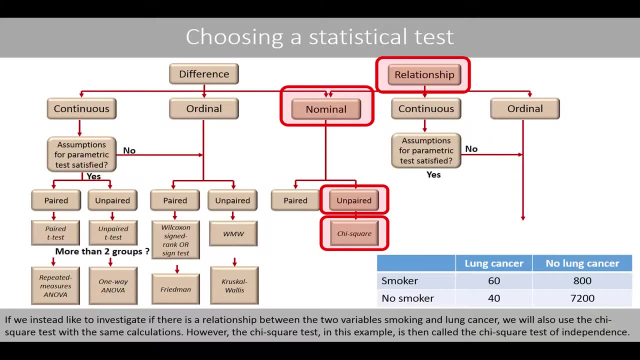 we can either use the Chi-square test of homogeneity or the two-proportions Z-test. If we instead like to investigate if there is a relationship between the two variables, smoking and lung cancer, we will also use the Chi-square test with the same calculations. 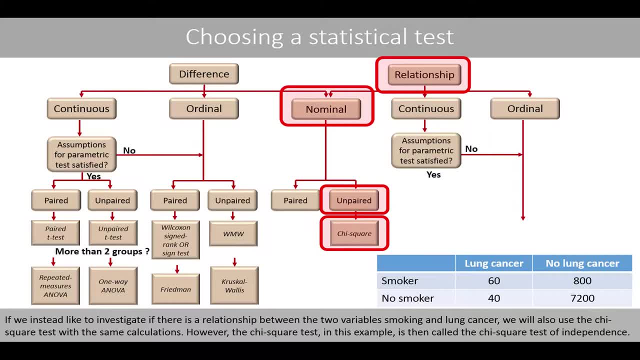 However, the Chi-square test in this example is then called the Chi-square test of independence. Fisher's test can be used as an alternative to the Chi-square test if one or more cells in the continuity table has an expected frequency that is less than 5.. 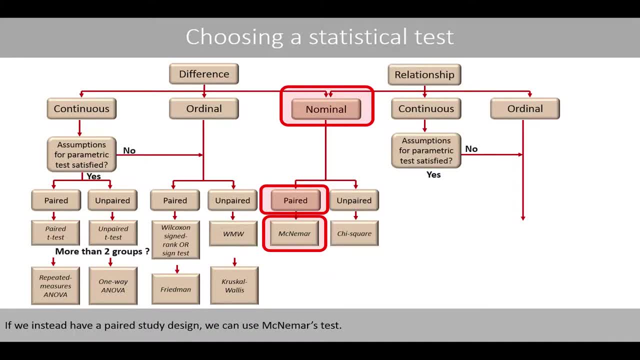 If we instead have a paired study design, we can use McNemar's test. Cochrane's Q-test can be seen as an extension on the McNemar's test if there are more than two treatments. Remember that the Chi-square test. 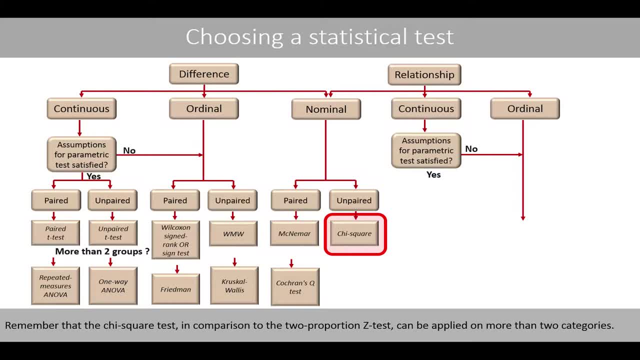 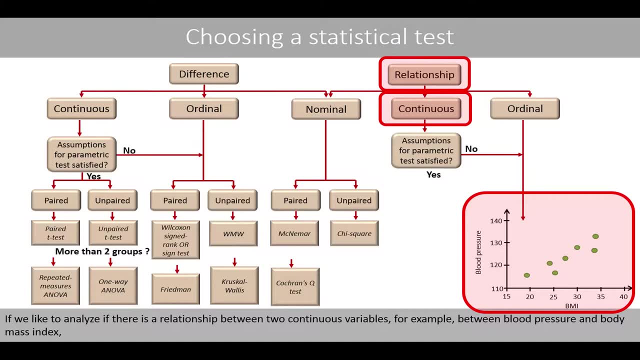 in comparison to the two-proportions Z-test can be applied on more than two categories. If we like to analyze if there is a relationship between two continuous variables, for example between blood pressure and body mass index, we could use the Pearson correlation if we fulfill its assumptions. 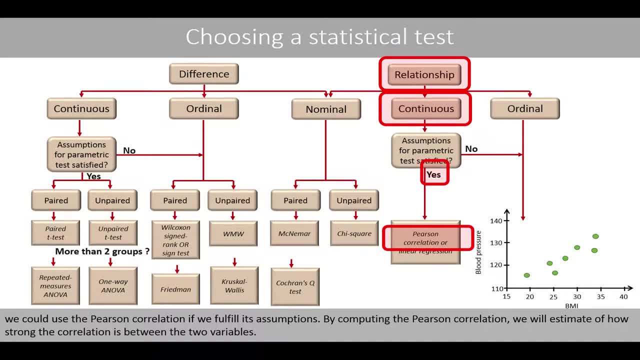 By computing the Pearson correlation, we will estimate how strong the correlation is between the two variables If we instead would like to, for example, predict the blood pressure given a certain body mass index or estimate how much the body mass index affects the blood pressure. 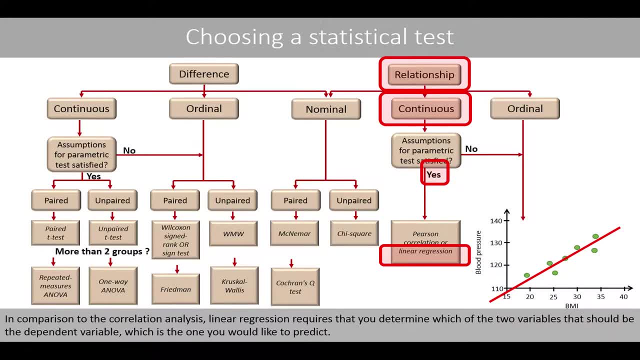 we could use linear regression In comparison to the correlation analysis. linear regression requires that you determine which of the two variables that should be the dependent variable, which is the one you would like to predict In the case where we do not fulfill the assumptions. 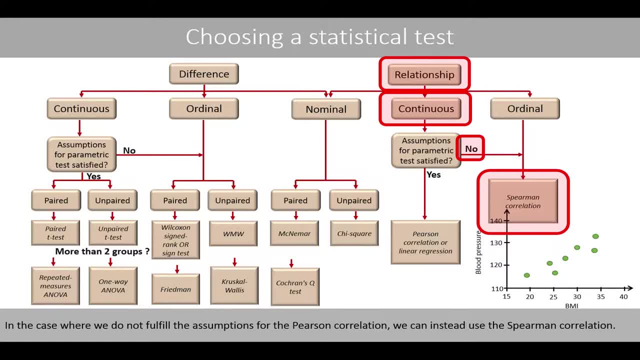 for the Pearson correlation. we can instead use the Spearman correlation. Also, if one or both variables have an ordinary scale, the Spearman correlation can be used. For example, we can test if there is a correlation between blood pressure and different age groups. 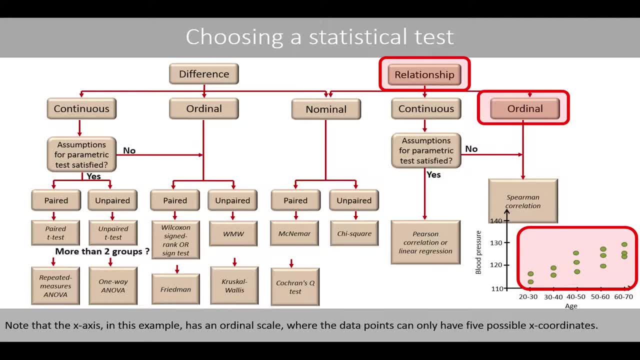 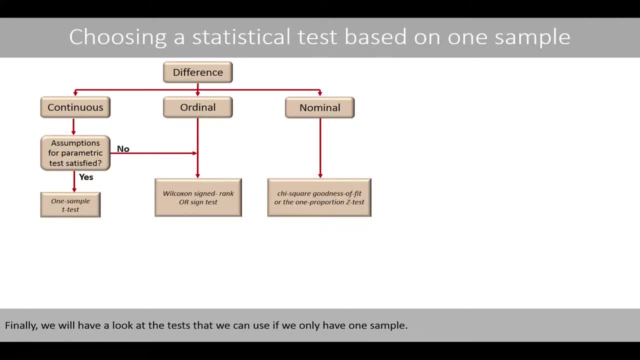 Note that the x-axis in this example has an ordinary scale, where the data points can only have five possible x-coordinates. Finally, we have a look at tests that can be used if we only have one sample. For example, let's say that we have measured. 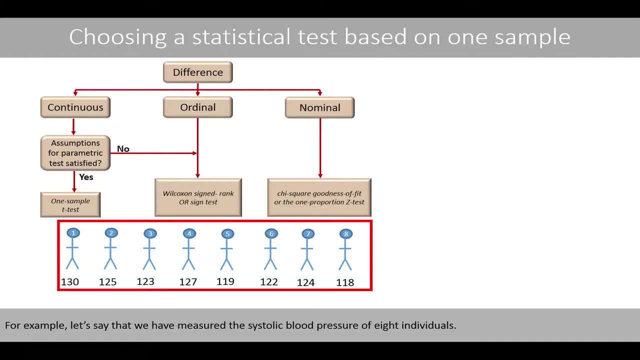 the systolic blood pressure of eight individuals. The mean systolic blood pressure of these eight individuals is 123.5.. If we'd like to compare if this blood pressure differs from the population mean or hypothesized mean, we can use a one-sample test. 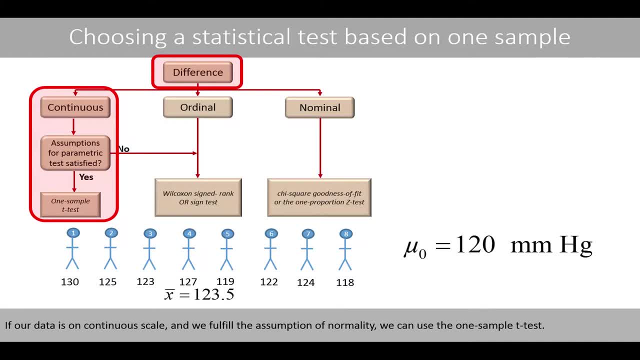 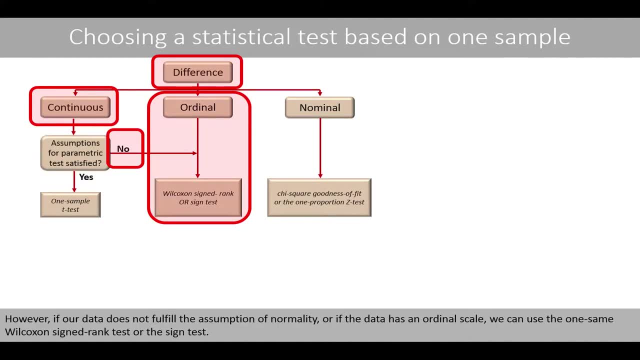 If our data is on continuous scale and if we fulfill the assumption of normality, we can use the one-sample t-test. However, if our data does not fulfill the assumption of normality or if the data has an ordinary scale, we can use the one-sample Wilcoxon sign-rank test. 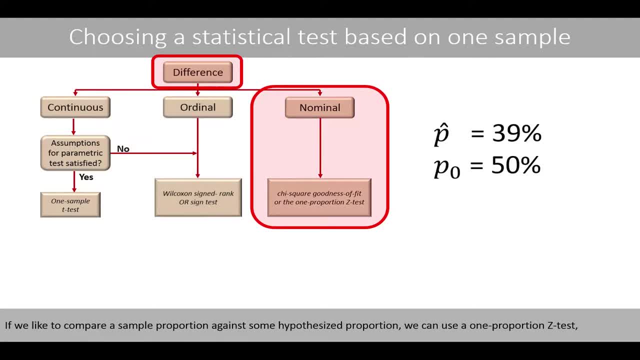 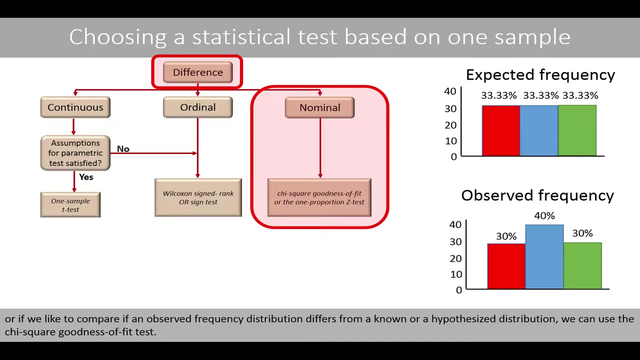 or the sign test. If we'd like to compare a sample proportion against some hypothesized proportion, we can use a one-proportion z-test. Or if we'd like to compare if an observed frequency distribution differs from a known or hypothesized distribution, 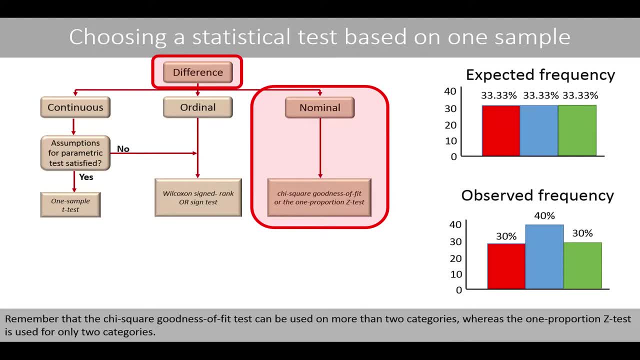 we can use the chi-square goodness of fit test. Remember that the chi-square goodness of fit test can be used on more than two categories, whereas the one-proportion z-test is used for only two categories. We'll now have a look at some simple examples. 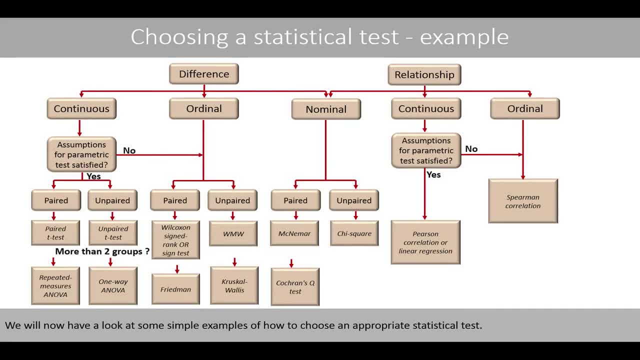 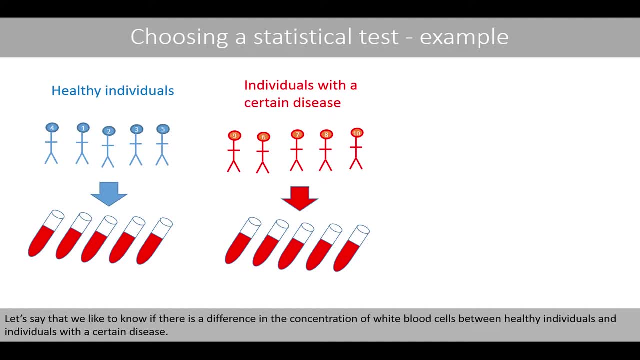 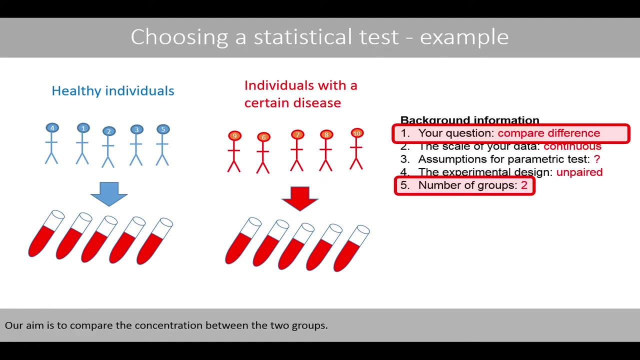 of how to choose an appropriate statistical test. Let's say that we'd like to know if there is a difference in the concentration of white blood cells between healthy individuals and individuals with a certain disease. Our aim is to compare the concentration between the two groups. 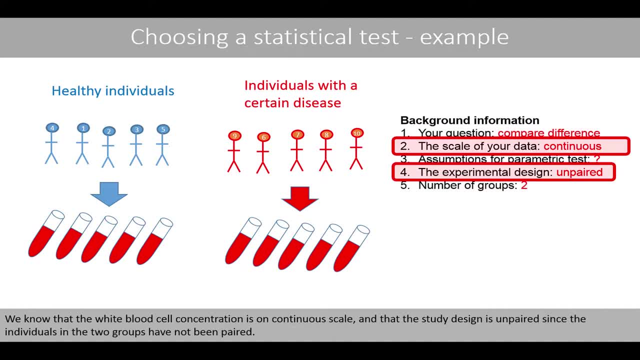 We know that the white blood cell concentration is on continuous scale and that the study design is unpaired since the individuals in the two groups have not been paired. Note that it is impossible to randomly assign who should be in the healthy group and who should be in the diseased group. 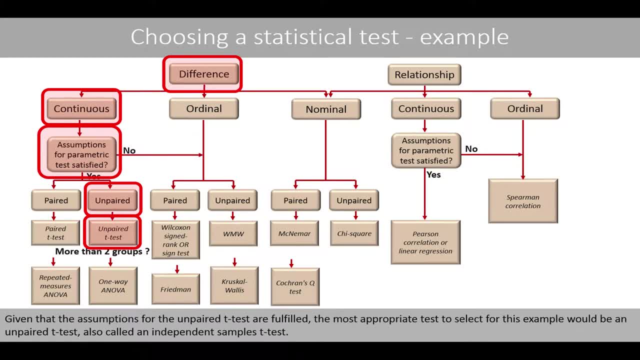 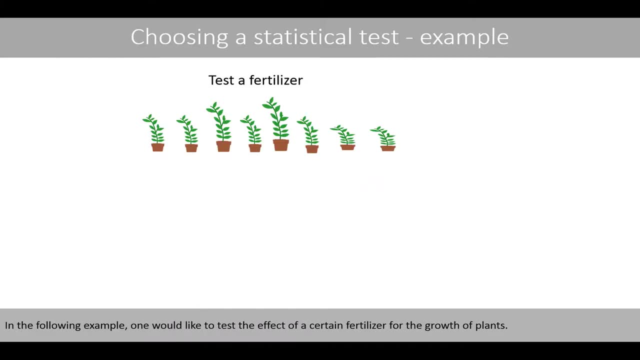 out of the ten participants. Given that the assumptions for the unpaired t-test are fulfilled, the most appropriate test to select for this example would be an unpaired t-test, also called an independent samples t-test. In the following example, one would like to test the effect of a certain fertilizer. 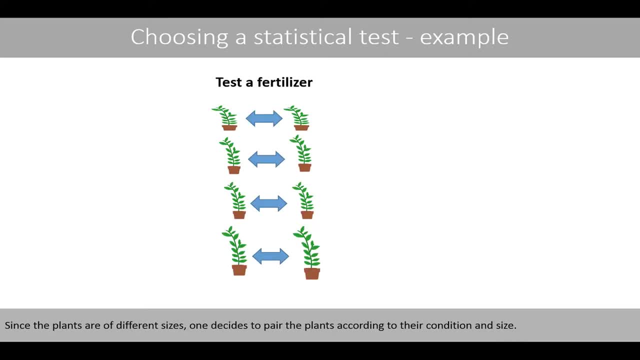 for the growth of plants. Since the plants are of different sizes, one decides to pair the plants according to their condition and size. One of the plants in the pairs is then given the fertilizer. The effect of the fertilizer is determined based on the number of factors. 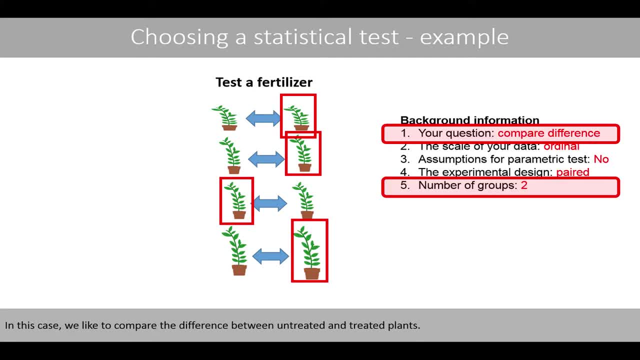 that is summarized in a scale from 1 to 10.. In this case, we like to compare the difference between untreated and treated plants. We have used the paired study design. A number of measures of the growth of the plants have been combined into a scale from 1 to 10,. 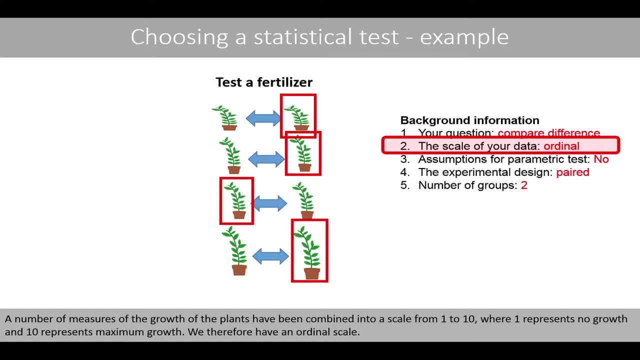 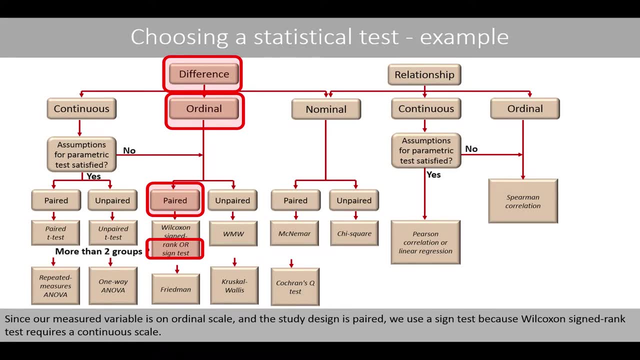 where 1 represents no growth and 10 represents maximum growth. We therefore have an ordinal scale. Since our measured variable is on ordinal scale and the study design is paired, we use a sign test because Wilcoxon sign writing test requires a continuous scale. 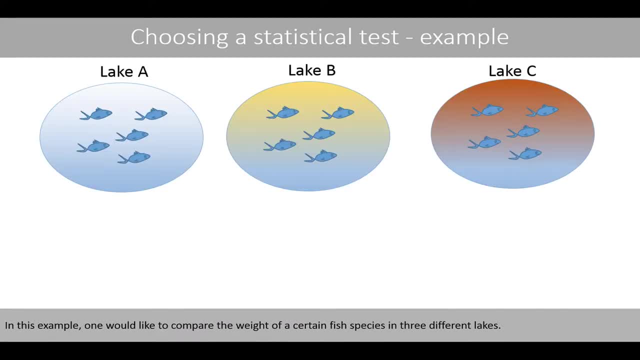 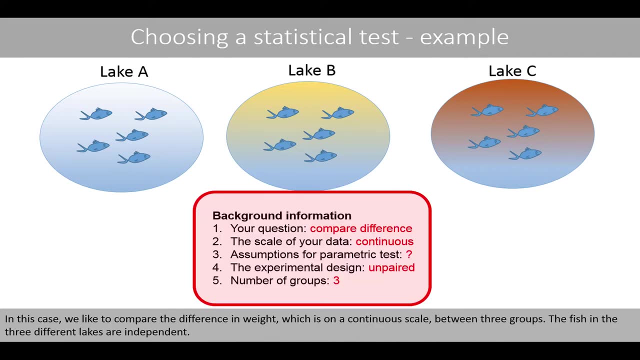 In this example, one would like to compare the weight of a certain fish species in three different lakes. In this case, we like to compare the difference in weight, which is on continuous scale, between three groups: The fish in the three different lakes. 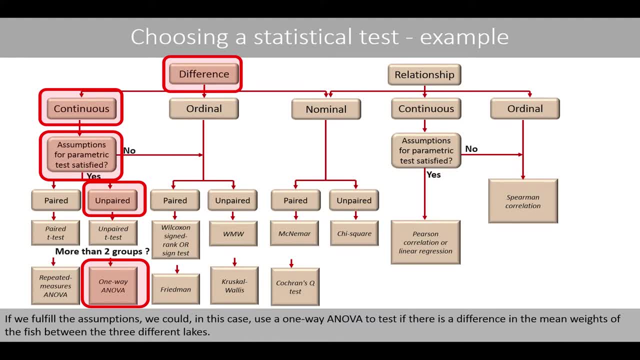 are independent. If we fulfill the assumptions, we could, in this case, use a one-way ANOVA to test if there is a difference in the mean weights of the fish between the three different lakes. If we do not fulfill the assumptions, we could consider using the Cascade-Wallis test. 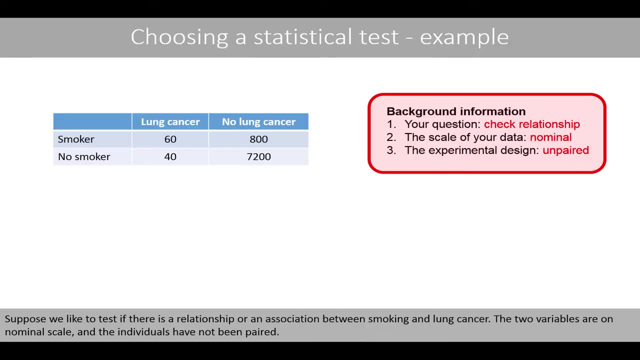 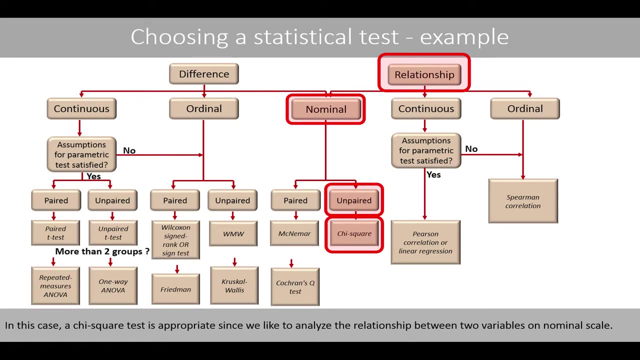 Suppose we like to test if there is a relationship or an association between smoking and lung cancer. The two variables are on numeral scale and the individuals have not been paired. In this case, a chi-square test is appropriate, since we like to analyze the relationship. 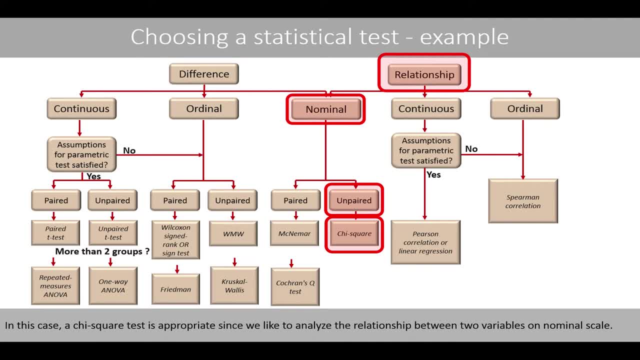 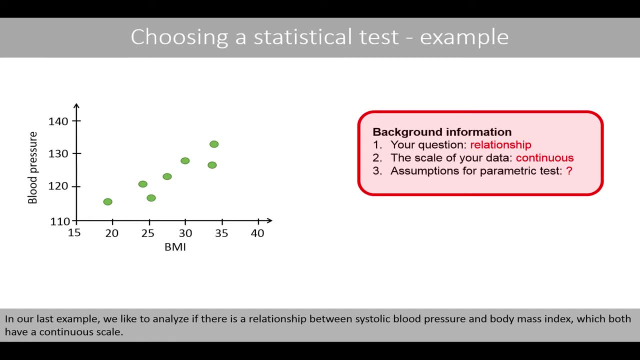 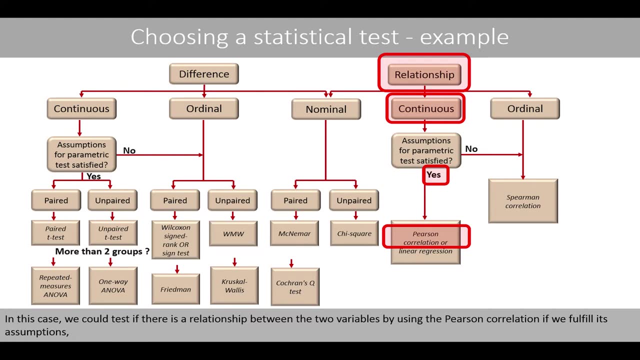 between two variables on numeral scale. In our last example, we like to analyze if there is a relationship between systolic blood pressure and body mass index, which both have a continuous scale. In this case, we could test if there is a relationship between the two variables. 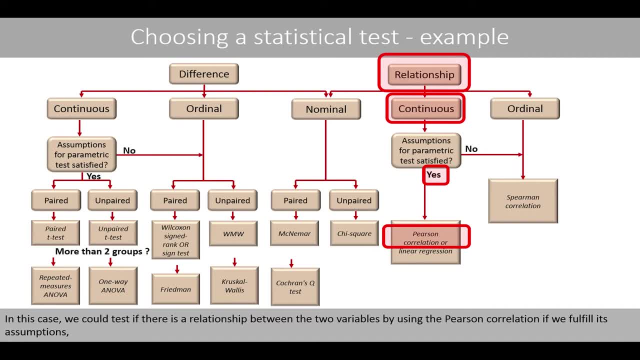 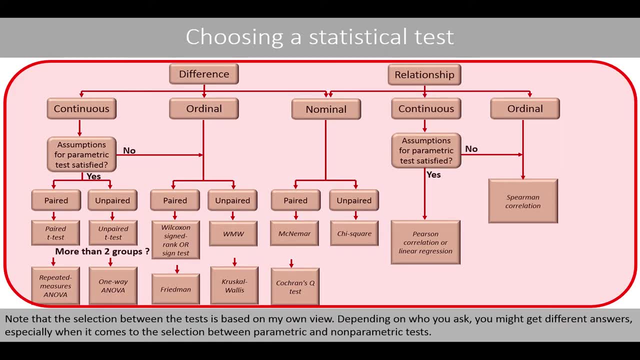 by using the Pearson correlation if we fulfill its assumptions, or the Spearman correlation if we do not fulfill the assumptions. Note that the selection between the tests is based on my own view. Depending on who you ask, you might get different answers, especially when it comes to the selection.